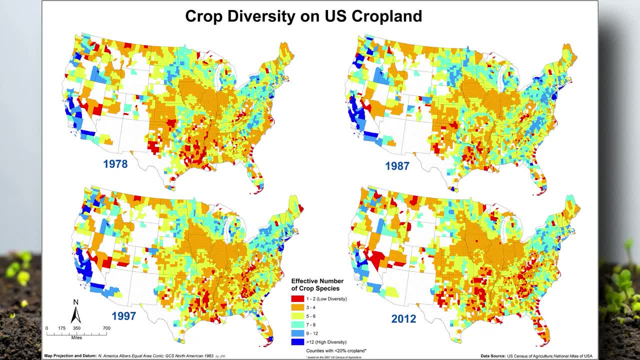 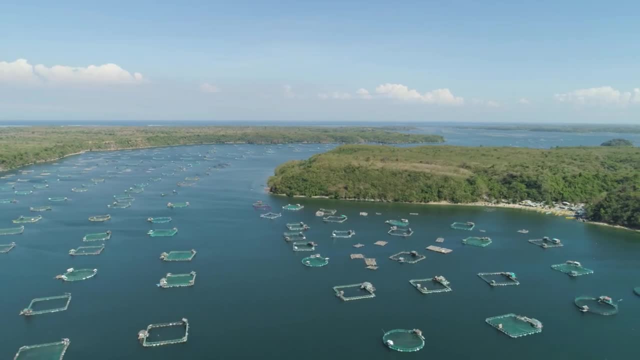 environmental concerns, as the amount of plant variance has significantly decreased over the years, as more farmers are using hybrid and GMO seeds for planting. This makes crops more susceptible to be completely wiped out by a disease. We can also see similar trends for livestock and fish, As aquaculture continues to be used. we can see markets now are only 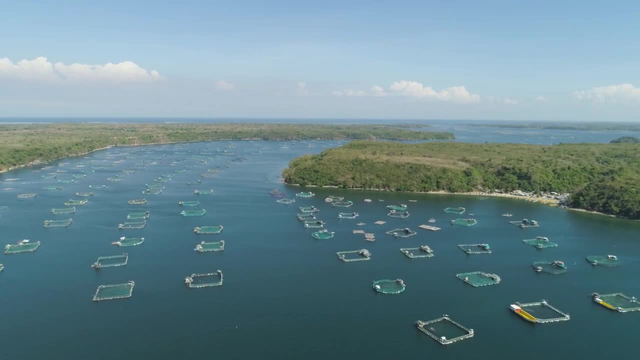 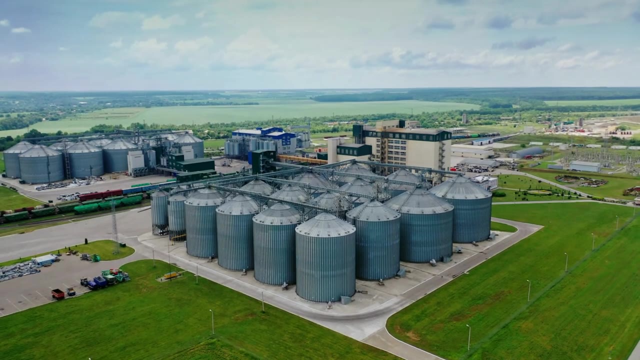 focusing on one or two species of fish. This allows them to specialize more and generate more profit. Today, thanks to the industrial food system, livestock animals now need to be the same size and weight In order to be able to be processed in plants. this has led to animals to now be fed food, that's 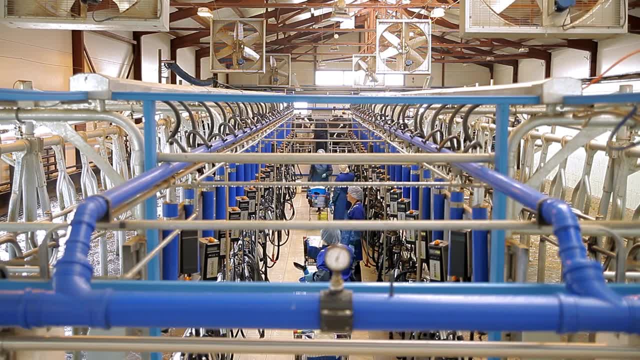 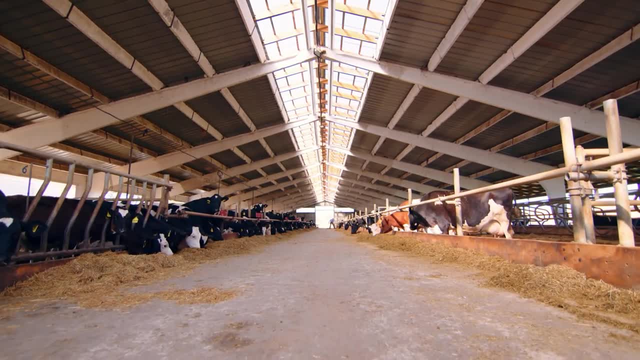 not part of their natural diets or be injected with growth hormones and antibiotics to make sure they're able to be the perfect size for processing. This has also led to concerns about antibiotics becoming less effective due to overuse in our livestock. If we turn our focus to the 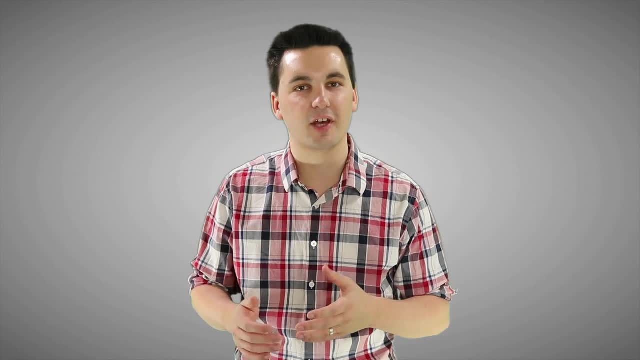 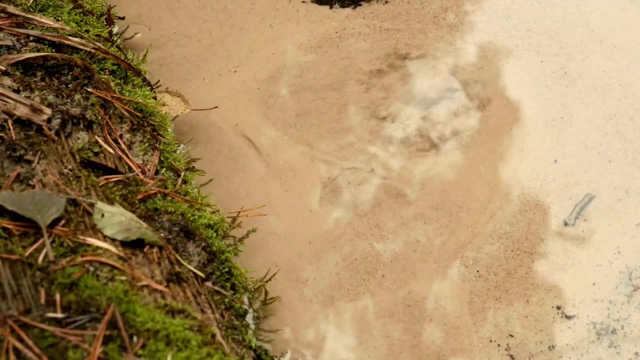 fields, we can see farmers often use chemical fertilizers and pesticides to help grow their crops. Unfortunately, these chemicals often run off into the local lakes, ponds and oceans. This can impact not only the ecosystems, which hurts local wildlife, but also impacts 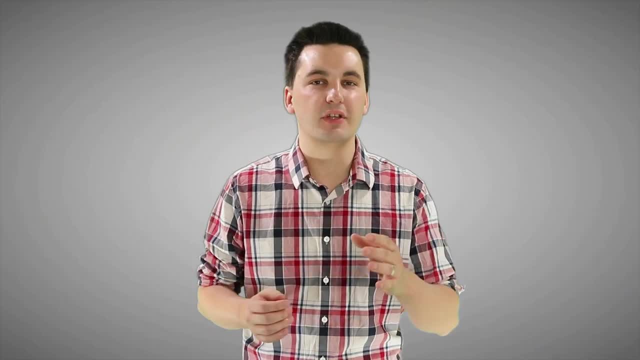 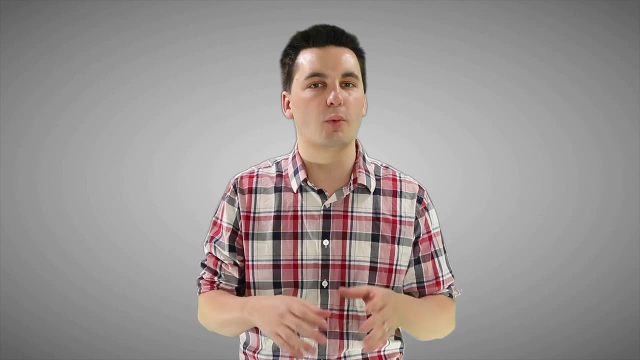 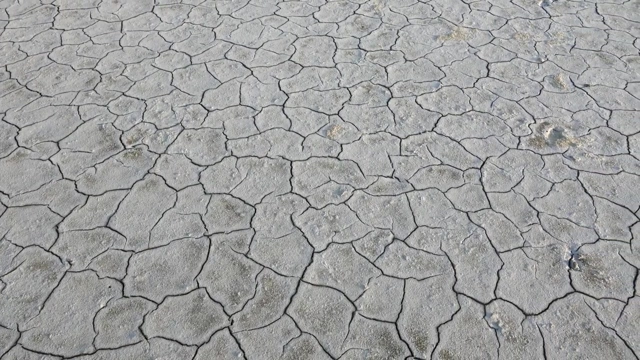 water sources for human consumption. We can also see the negative impact of irrigation practices, as farmers can unintentionally deplete local aquifers, rivers and streams. This also could lead to more water runoff, which would increase water pollution in the region. We can also see soil salinization occur due to water evaporation, especially in semi-arid. and arid lands. Even when food's been harvested, processed and shipped to consumers, we still see food waste and it can lead to food spoiling. Many countries often lack infrastructure needed to keep food from spoiling or transportation systems to get food to the right market on. 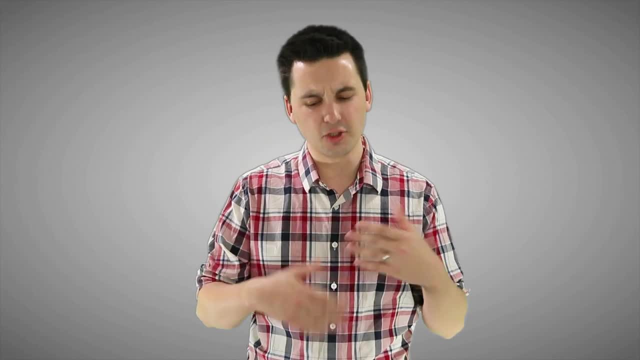 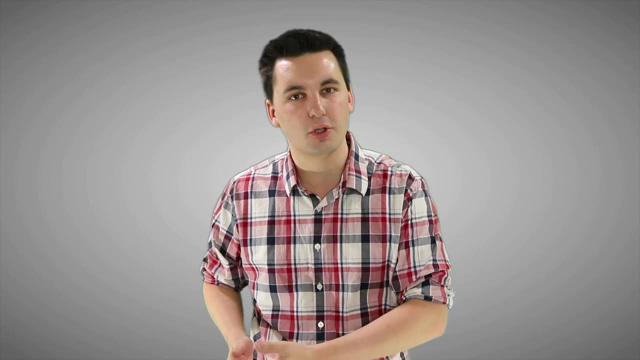 time, As our food system continues to become more industrialized, we continue to struggle with new problems, such as the food miles problem, which looks at how many miles food must travel from when it's produced to the consumer. The larger that number is, the more. 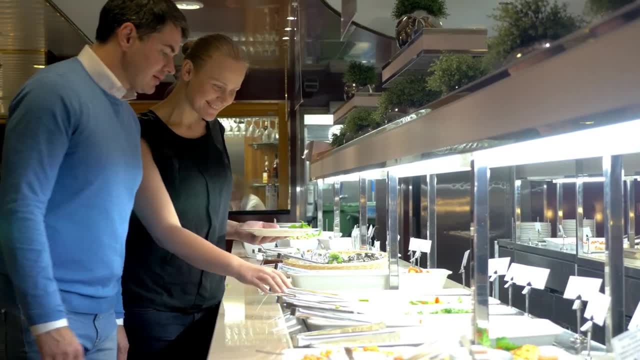 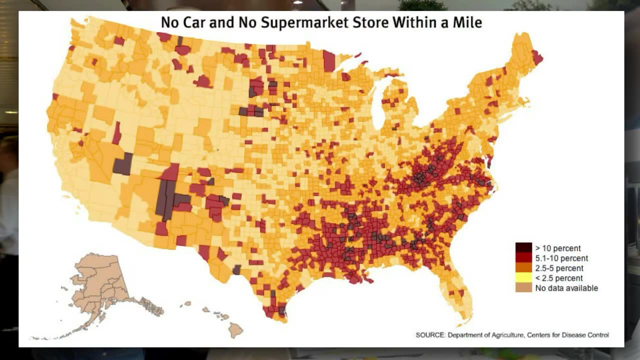 inefficiencies we have Today. we can also see how people's food choices are being influenced by changes in their food choices. For example, in the United States, food choices are being our agricultural practices. Households that are located in urban areas are more likely to live in. 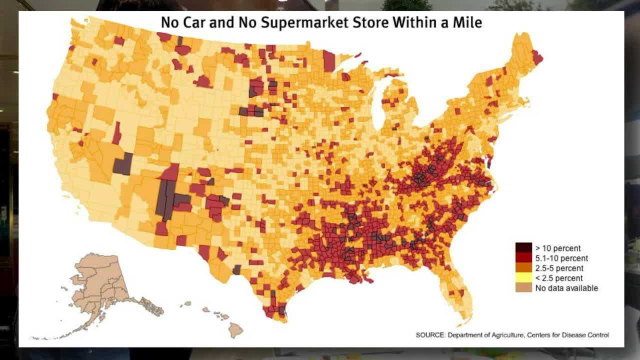 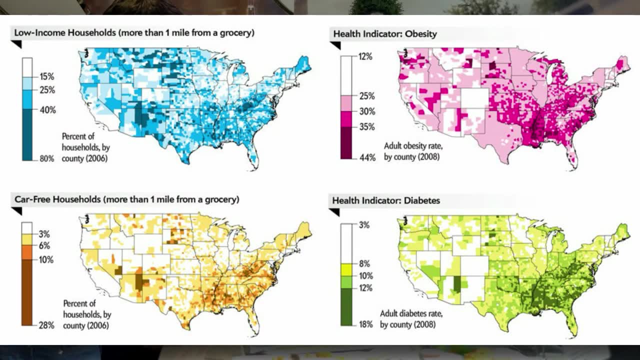 a food desert. People who live in a food desert do not have access to healthy food and often do not have access to a traditional grocery store or supermarket. People who live in food deserts are more likely to get their food from a convenience store or fast food restaurant and are more likely. 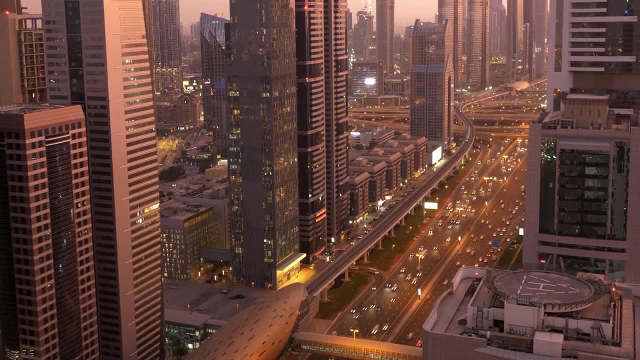 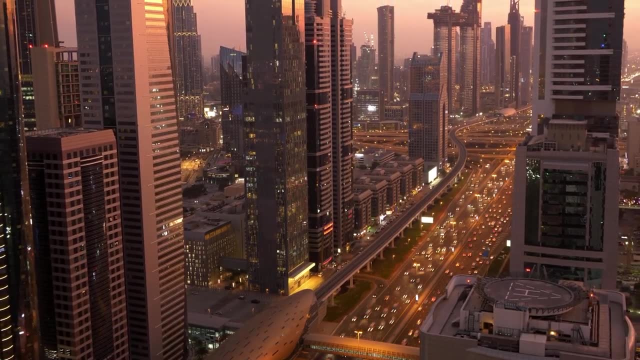 to have problems with obesity and diabetes. And as cities continue to grow due to urban sprawl, we continue to see agricultural lands lost, which can lead to a rise in food deserts and also increases the food miles problem. However, we can also see new urban farms that are being created. 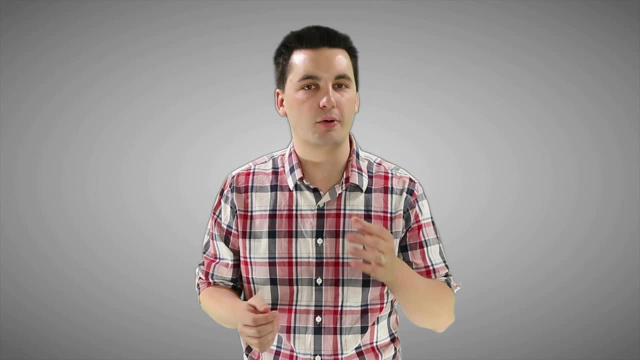 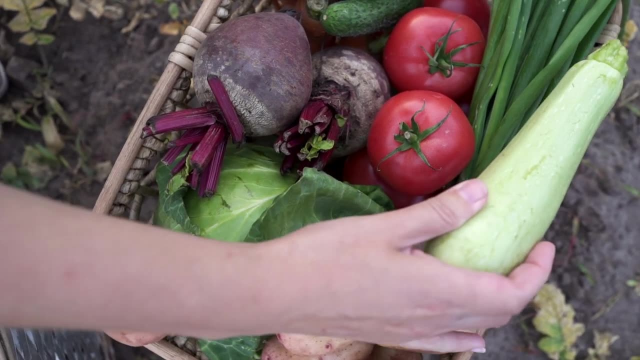 not only to help create more sustainable cities, but also to help counter food deserts. We could also look at the impact of community support agriculture, or CSA. This is when farmers sell some of their crops and products to local consumers who have agreed to buy the products. 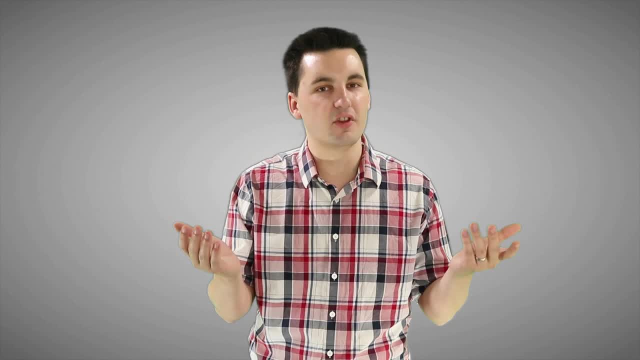 throughout the year. This not only helps support local farmers, but it reduces the amount of food miles of crops. This is when farmers sell some of their crops and products to local consumers who have agreed to buy the products throughout the year. This not only helps support local farmers. 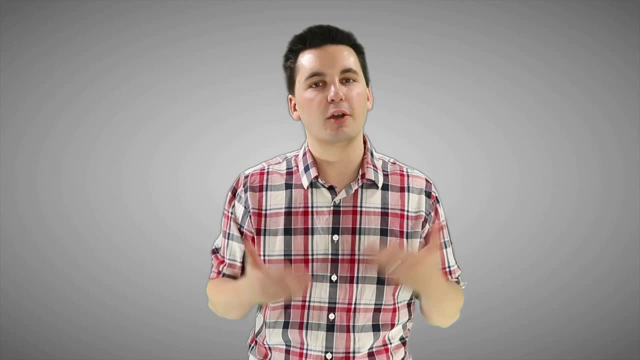 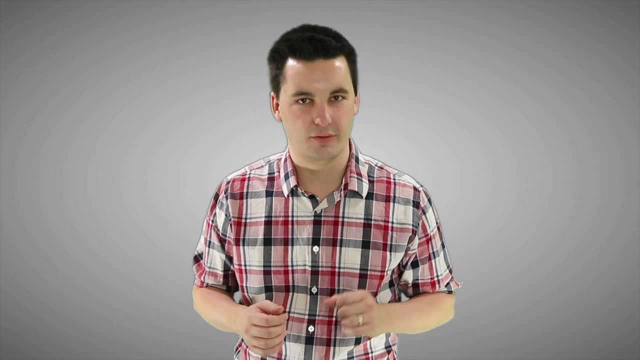 this allows farmers to use more environmentally safe practices and it reduces the amount of fossil fuel used to transport crops. Now, so far throughout this video, we've talked about a lot of negative things going on in the field of agriculture, but there's also some positive trends. Recently, we've seen consumers 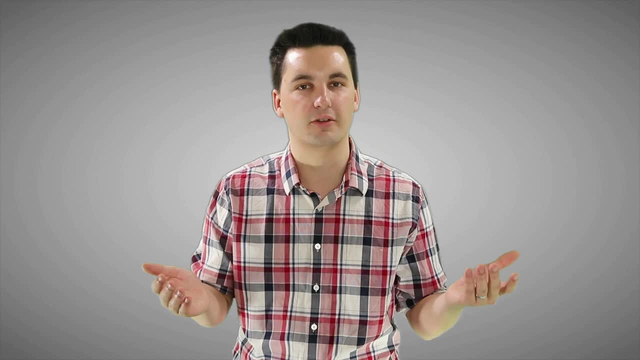 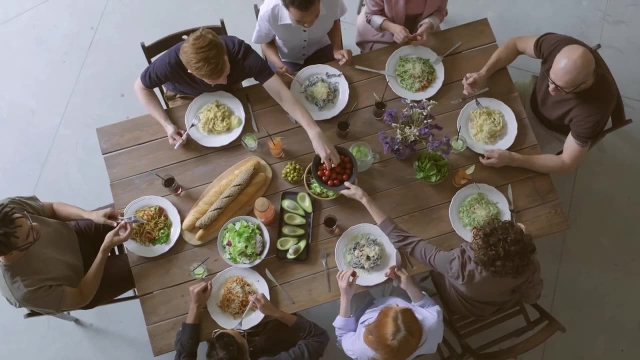 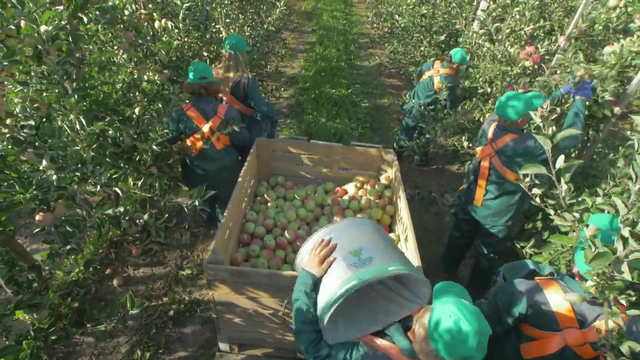 demand sustainable practices and healthier food options. More people today are wanting to eat chicken, rice, cheese and other healthier options. We have governments now putting policies in place to protect local environments and there's a greater focus on the international market. For example, today we've seen a rise in the organic food market. Organic farms are farms. 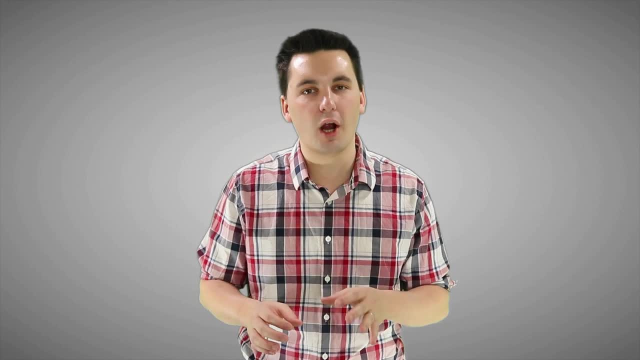 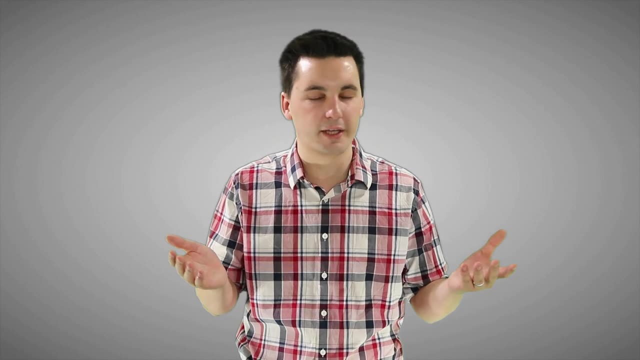 that don't use chemicals. They try to reduce the amount of water they're using and they use sustainable practices to help protect their natural resources. Livestock being raised on an organic farm also do not use chemicals, antibiotics or growth hormones, which can reduce. 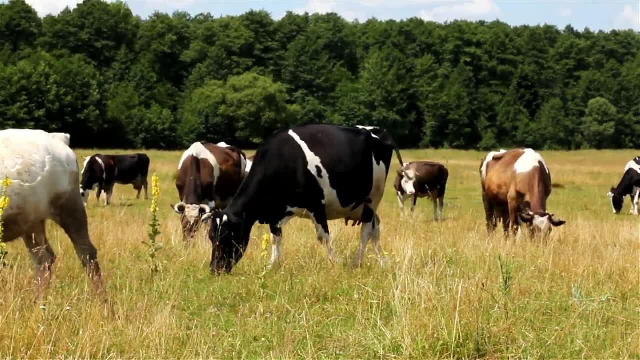 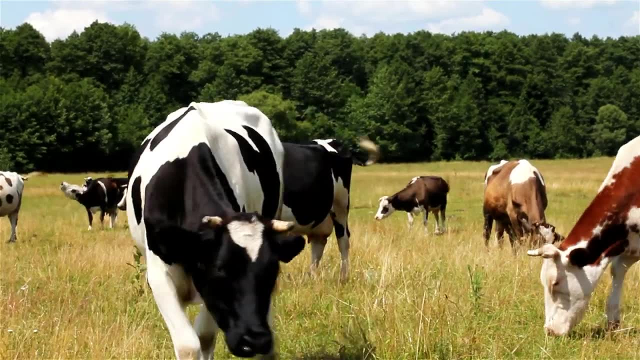 different negative impacts on the environment and the consumer's health. Livestock here will often also be free-range, which allows the animals to be able to live on their own, and they can also be able to live on their own for a longer period of time. For example, today we've seen a rise in 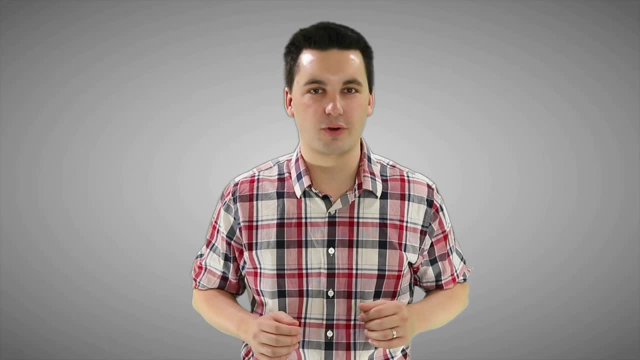 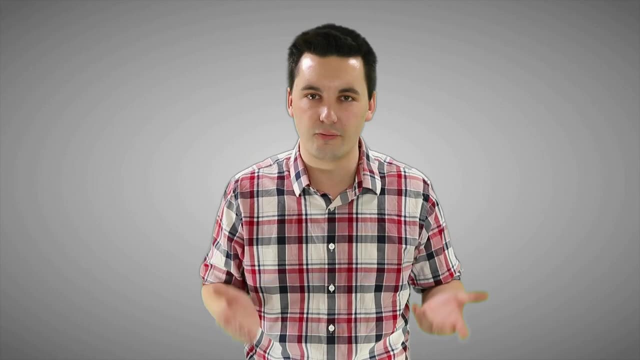 the amount of water they're using, which allows the animals to live in more of a natural environment. Recently, we've also seen a push for fair trade. Here, consumers can purchase products and food directly from the people who created them or the farmers who grew the food This allows for. 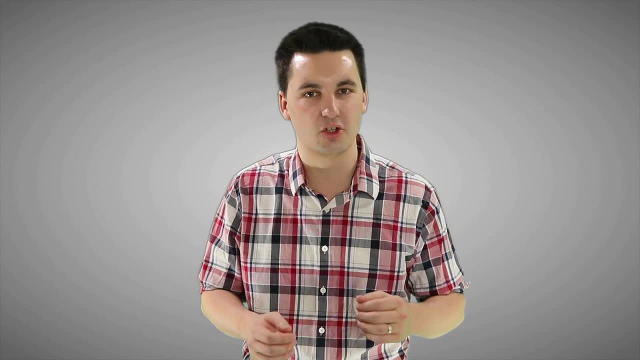 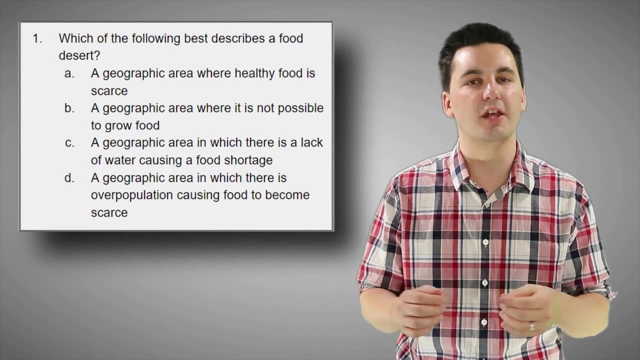 these people to get more of the profit. It also allows them to have better working conditions compared to if they worked for a multinational corporation. Our agricultural system today is complex, and we can see that all of our decisions do have consequences. Some of them are positive.